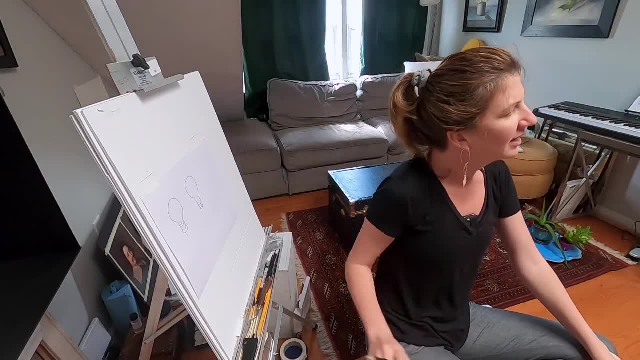 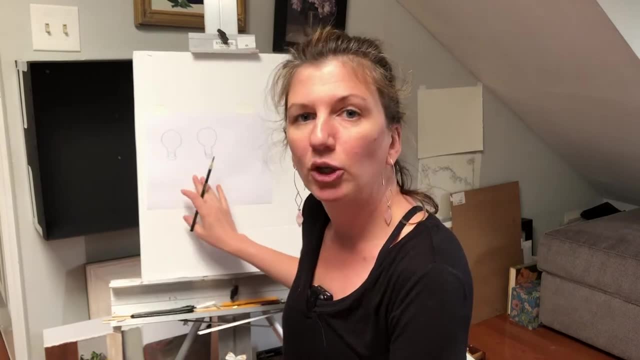 with paper. The lightest value that we can get on our paper is the color of the paper itself, But if you hold up a piece of white paper next to a light bulb, this paper will look so dark by comparison. Light also has a color, Even though it's really really. 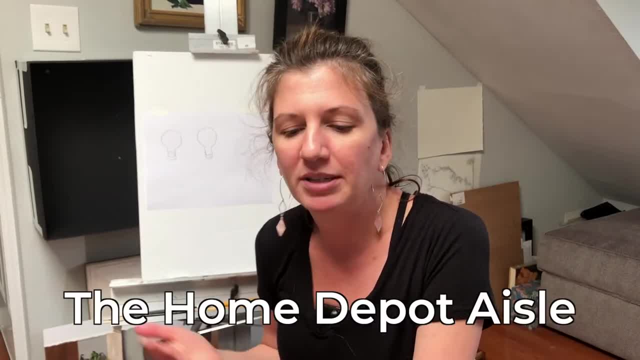 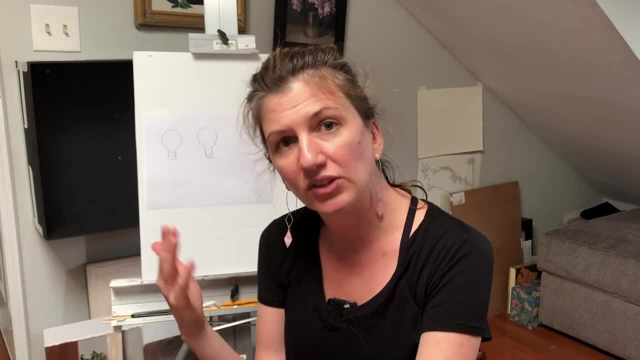 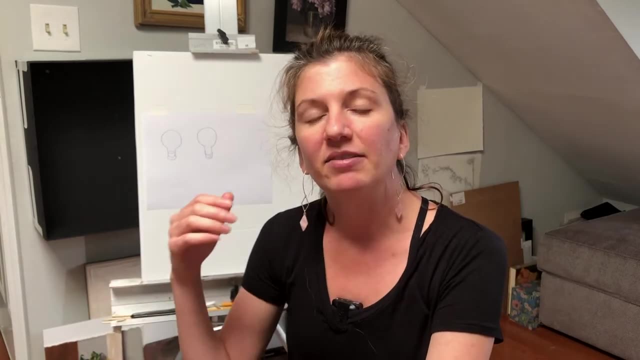 bright. you'll notice if you go to the grocery store or the Home Depot aisle or whatever. you'll see light bulbs and they have warm light, cool light, right. What they're talking about is the hue, So they have blue light and yellow light and orange light And it makes the room feel. 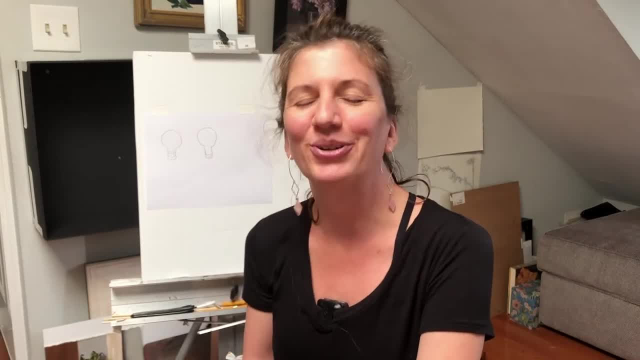 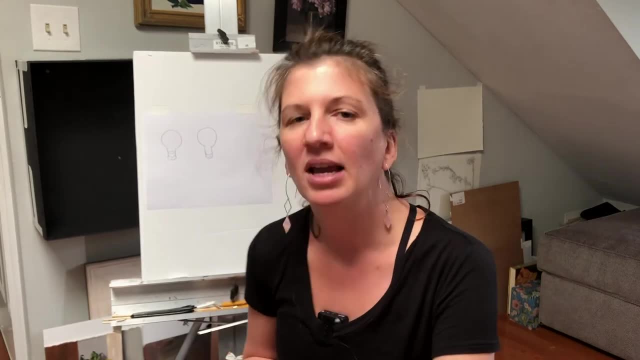 differently. If you've ever been in a light, if you've ever been in a room full of warm light, it tends to feel comfortable. If you have a room full of cool light, it tends to feel edgy and modern, And so you can see that both of those lights are so bright that we can't paint them, even if we. 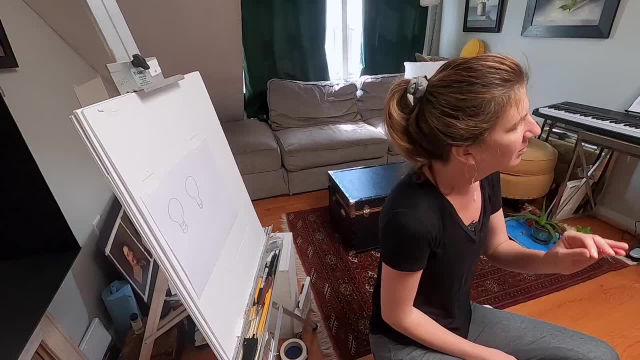 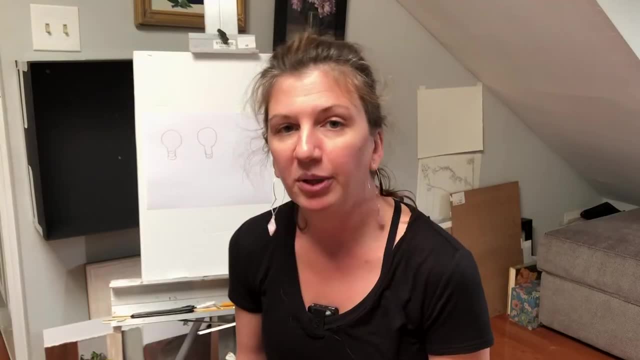 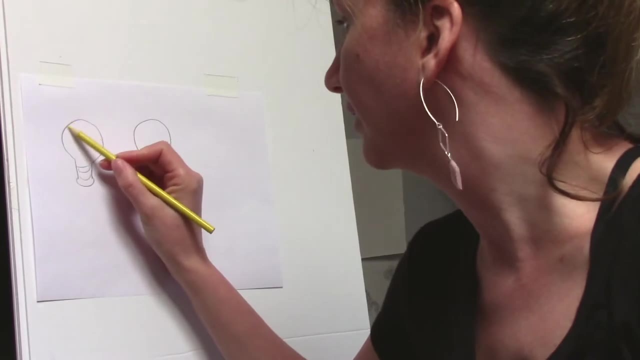 wanted to, But they also have color. Sometimes you have to choose between the chroma, the intensity of the color and the value, how light or dark something is. For example, if I want to show that light bulb number one here is yellow light, I'm going to go ahead and fill it in with yellow to. 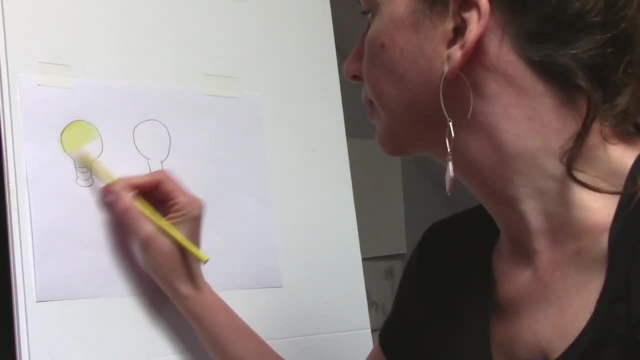 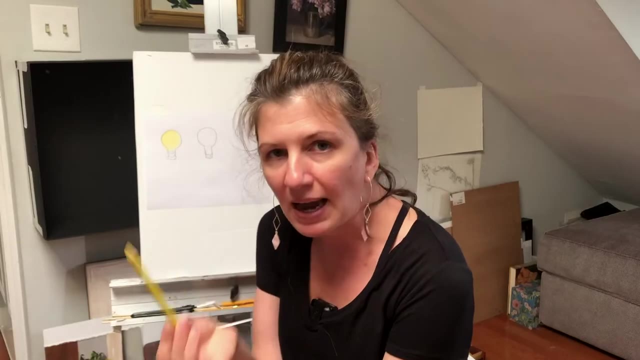 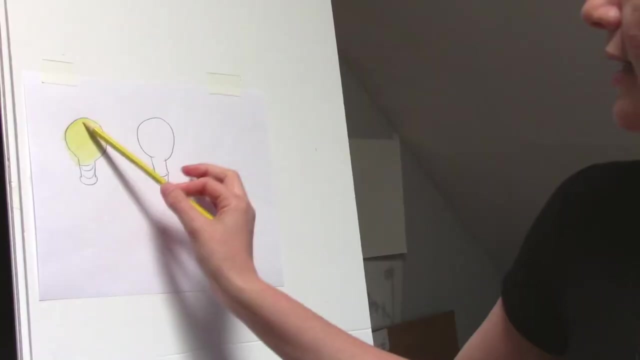 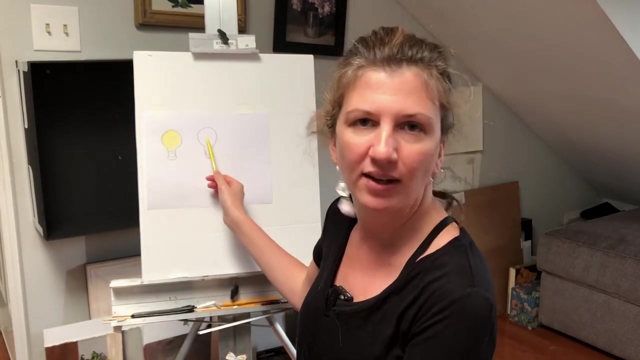 represent the hue, yellow, Yellow light. And this is not just any yellow. This is the most chromatic yellow I have. This is the most intense yellow in my colored pencil box. But this chroma- because it has a lot of chroma, it actually feels brighter to us than the one that's on the white piece of paper. 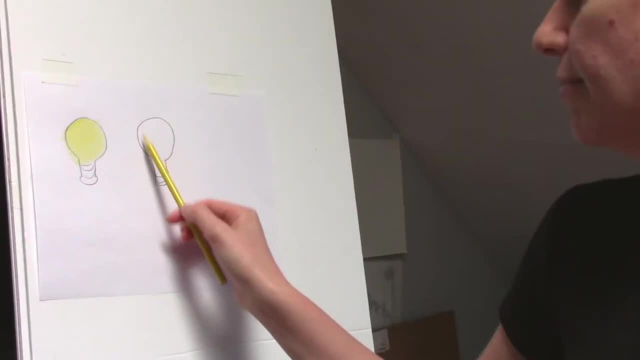 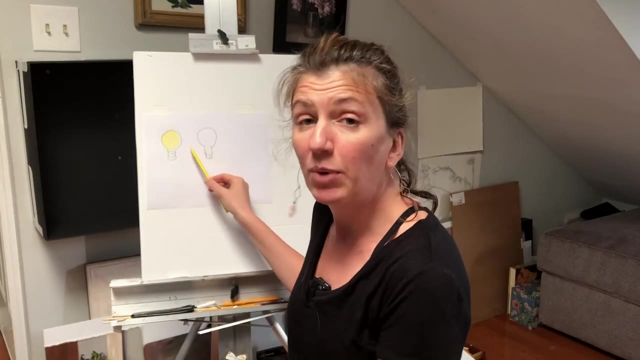 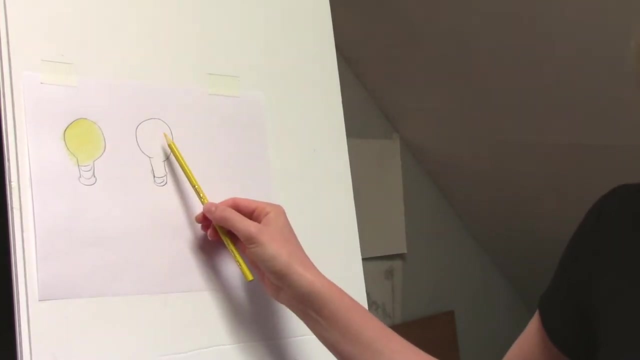 If you observe carefully, you'll notice that the white piece of paper is a lighter value than this yellow. This yellow is darker than the white. If you're painting something that's very bright and chromatic, you have to choose between the chroma and the value. Light bulb two. we'll call this light bulb two and this light bulb one. 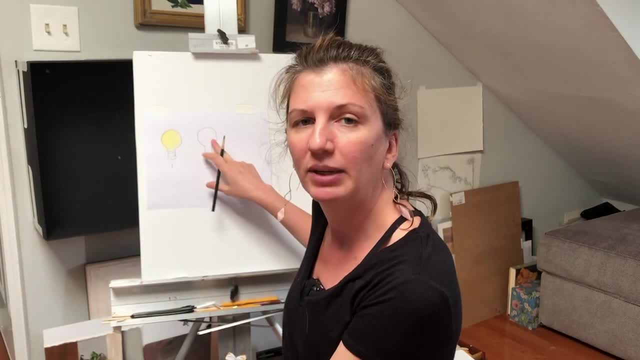 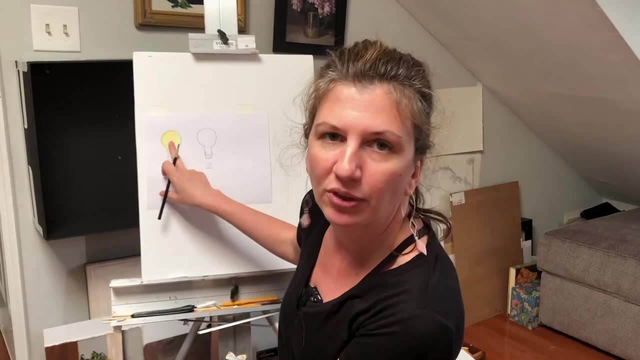 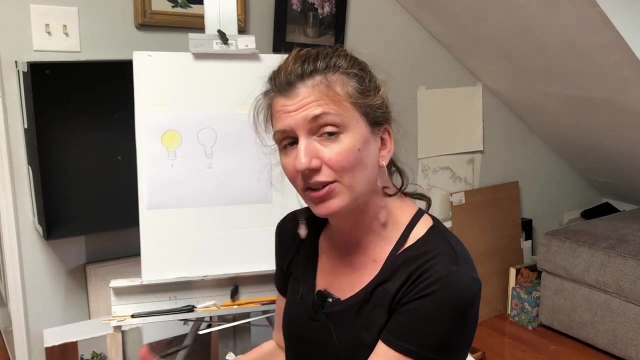 Light bulb two is choosing value. This is the lightest value we can have. Light bulb two is not sacrificing value to get the chroma. Light bulb one is going after the chroma, but it's sacrificing the value. This yellow is darker than the color of the paper. By understanding this,